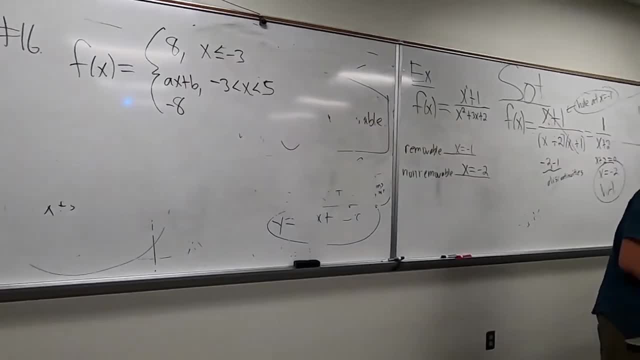 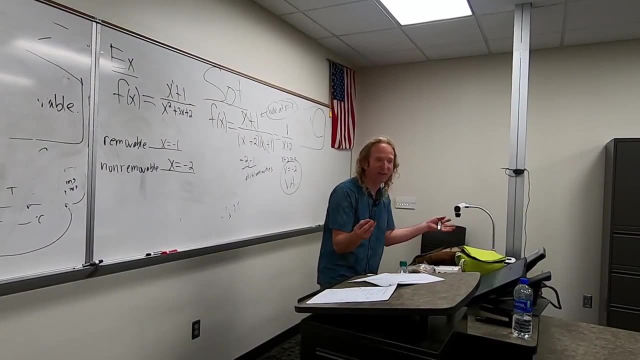 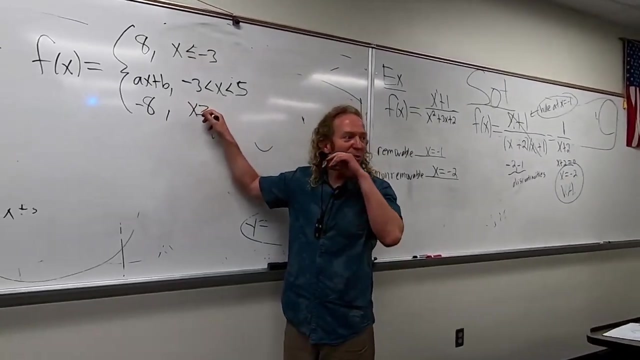 Who said that That's a point, Logan? No, it's good. No, it's fine. It doesn't affect my life. I don't know why it bothers me. It shouldn't Ax greater than or equal to 5.. 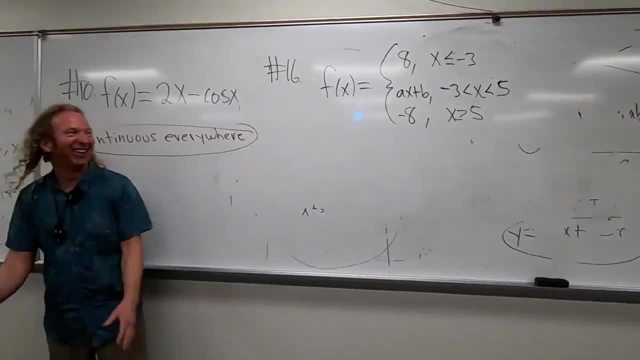 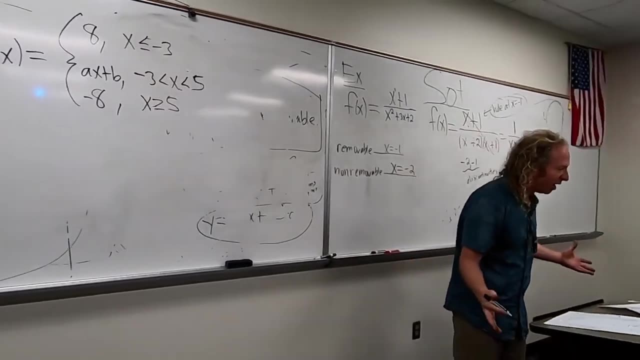 5. Give me the wrong one. No, it's fine, It's fine, It's good. I usually start losing points. Yeah, Yeah, Okay, Oh, what is the question? Find a and b so that the function is continuous everywhere. 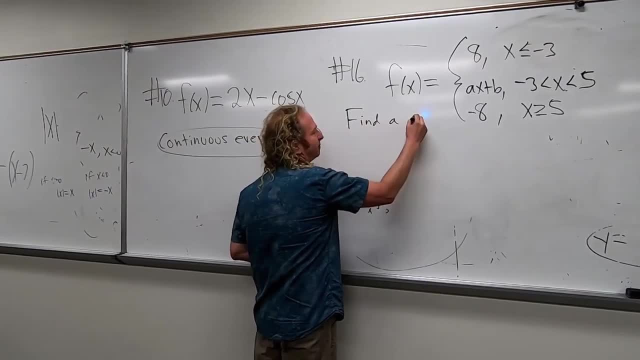 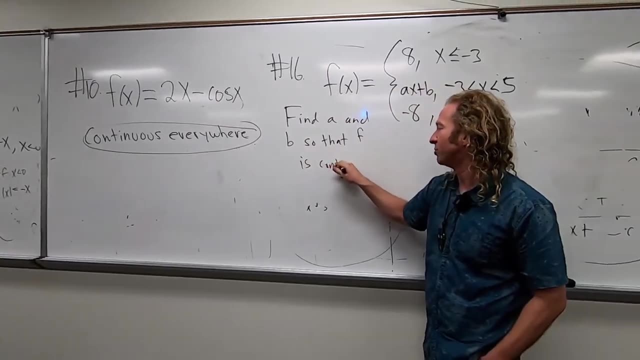 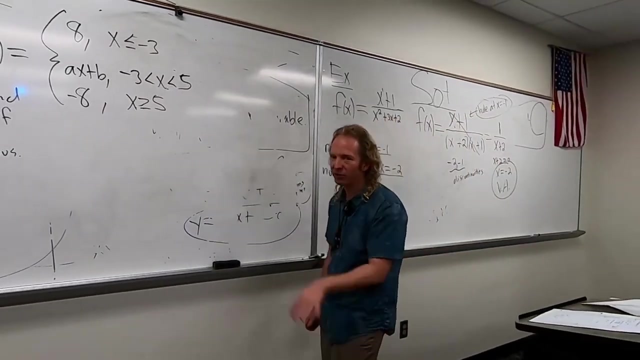 So find a, b so that f is continuous. I'm going to go really slow as we do this one. This is really tough Again. I was going to say something earlier and I forgot to say it In the videos there's a ton of videos on all of these questions. 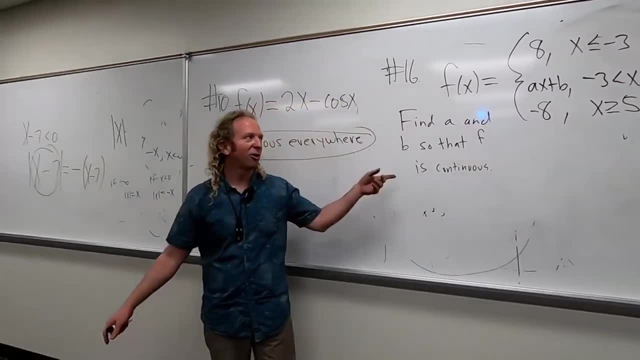 especially from this section, because I was going to make some yesterday and I clicked on the homework. I'm like, oh, I already have videos for all the hard ones, so I didn't make any. So this is all there if you click on the videos. 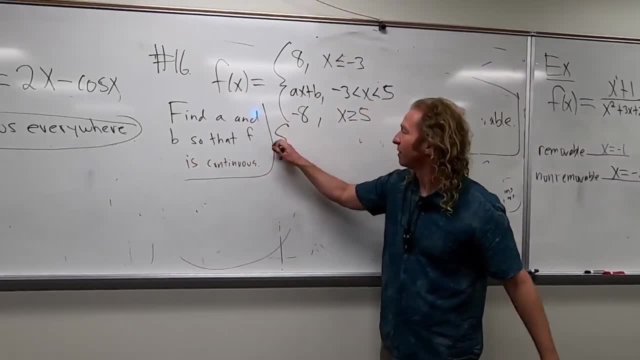 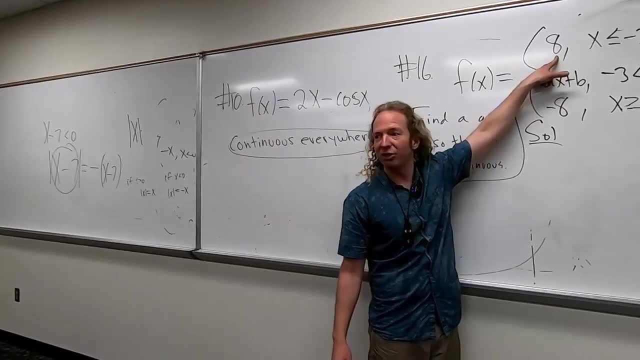 Okay, Because you'll probably get stuck. There's a bunch of these, So we have to make this continuous. This is a really weird problem because you have three functions right? So 8 is a horizontal line. By itself. it's continuous. 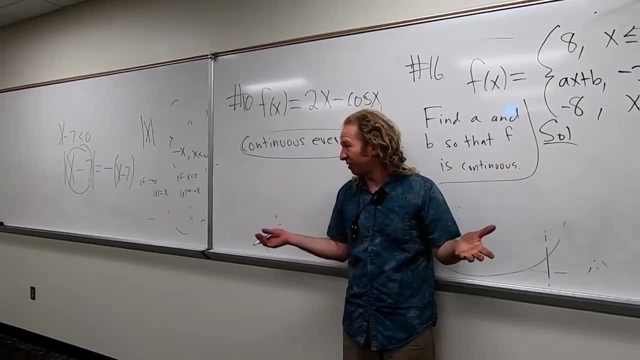 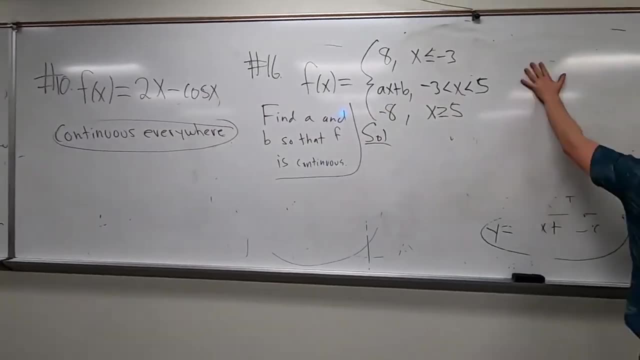 Ax plus b. Ax plus b is a straight line. It's kind of like mx plus b. By itself, it's continuous. Negative 8 is a horizontal line. By itself, it's continuous. So basically, the idea is that you have- I'm going to erase this, but I'll draw it. 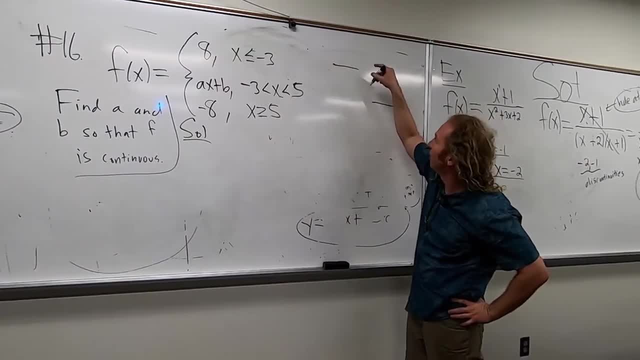 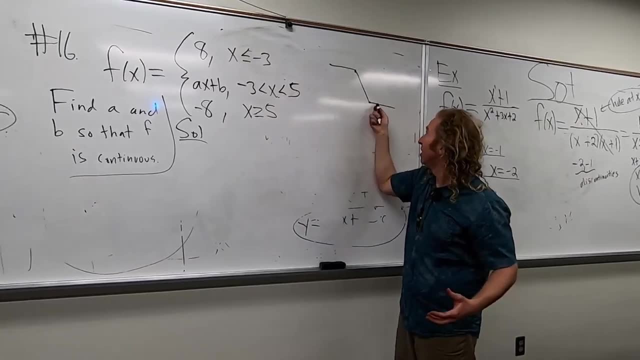 You have 8, negative 8, and then you have to find the line that connects them to make it continuous. That's the idea, right, Because this is 8.. This is negative 8.. And so ax plus b is somewhere here. 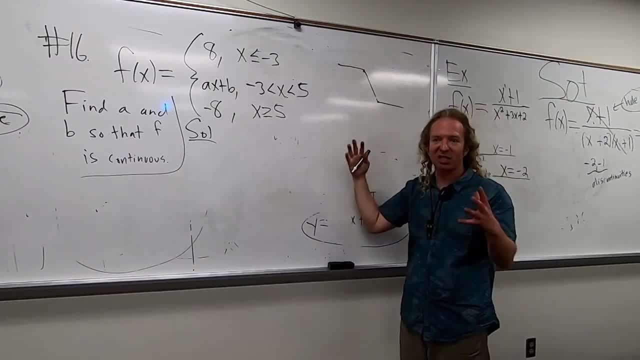 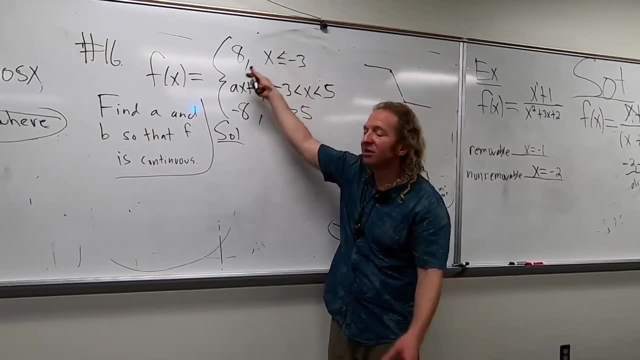 So you have to find a and b so that ax plus b actually connects these lines. That's a really deep way You're thinking about the problem. A simpler way is: this is continuous, this is continuous. this is continuous, But taken together as a whole, the function is probably not continuous. 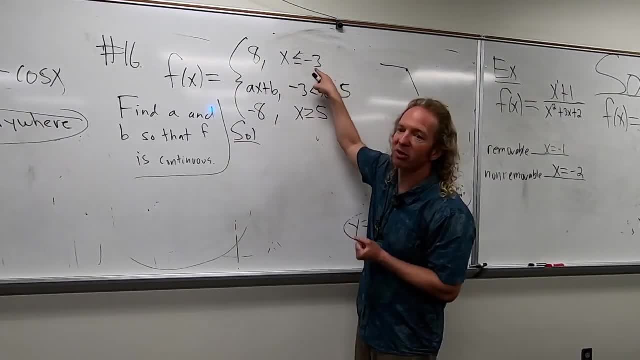 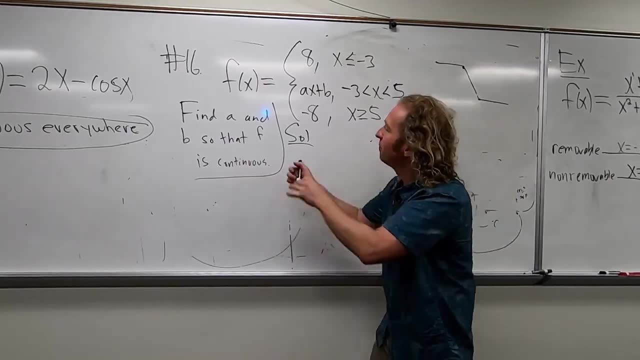 The only possible place that we can have a problem is at the end points. So negative 3 and 5.. So when you're doing these problems, just focus on the negative 3 and the 5. So you have to make sure that this is continuous at those numbers. 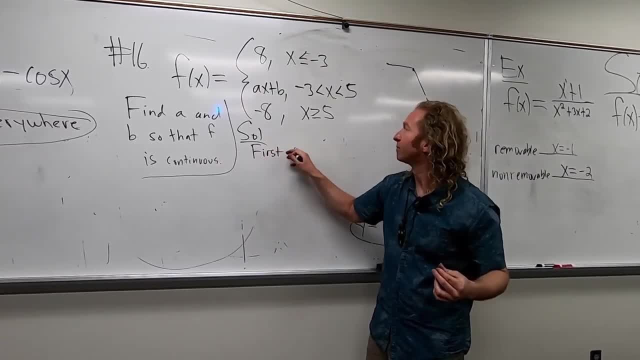 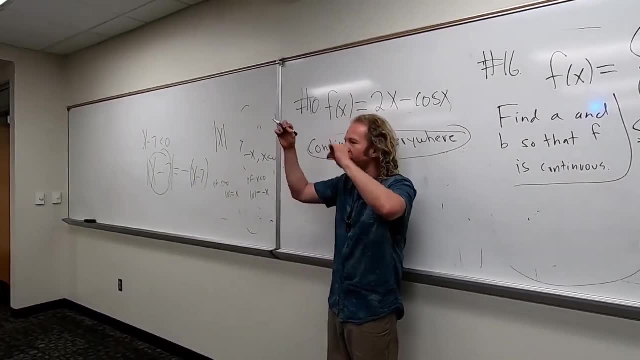 So first negative 3. So first let's do negative 3. So just do one at a time. So if you make it continuous at the end points, then basically you're connecting it right. Okay, So we had that definition of continuity. 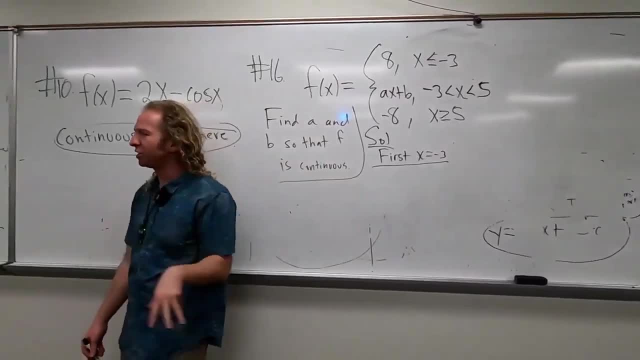 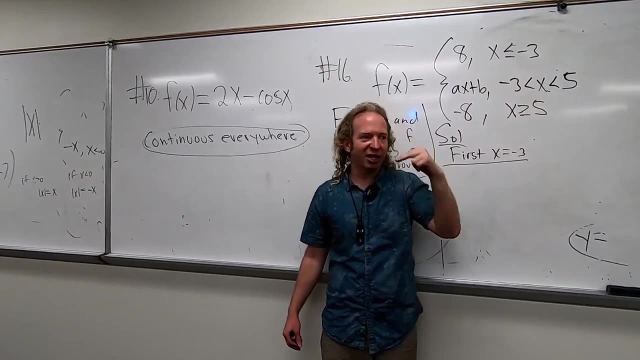 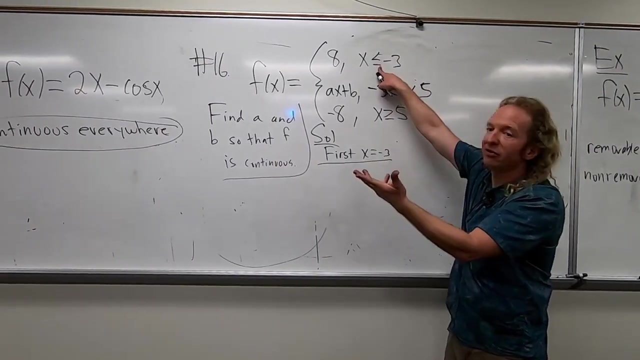 It had to be defined, The limit had to exist And that third condition as well. So here's a really cheap trick: Whenever you have these problems and you have less-thans and greater-thans, use the second condition. So in other words, to make sure that this function is continuous at negative 3, well, it's defined, obviously. 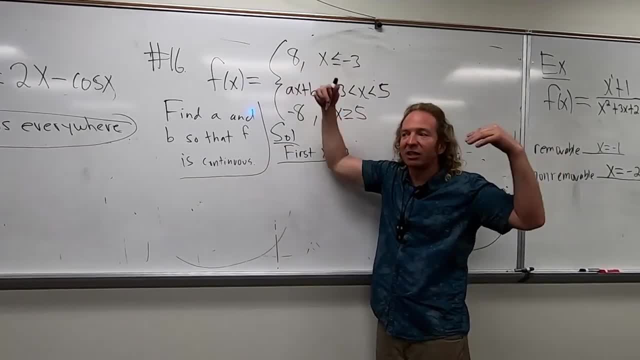 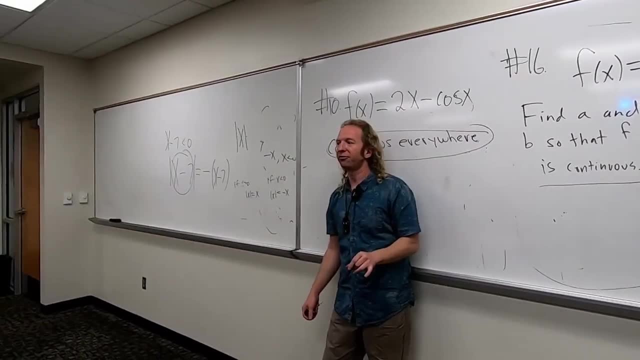 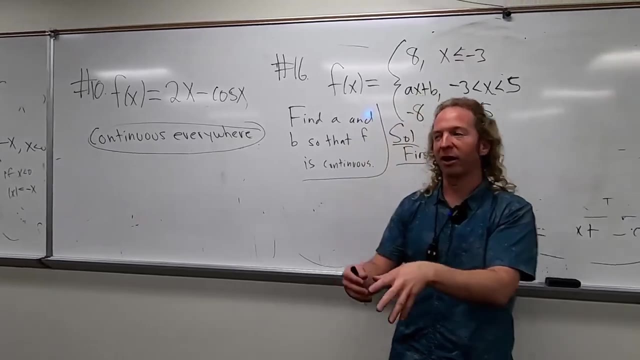 Because if you plug in negative 3, you get 8.. The second condition is that the limit has to exist. For a limit to exist, it has to exist from the left and from the right. So because we have less-thans and greater-thans, this problem allows us to work that way. 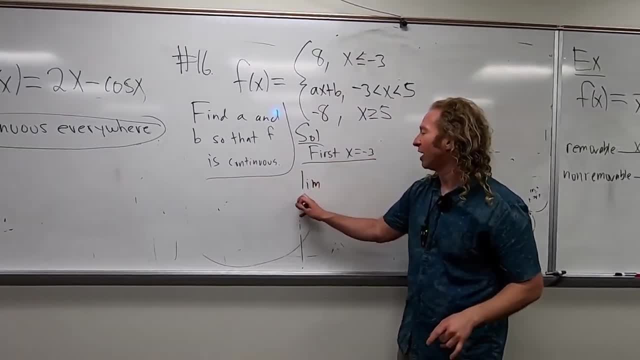 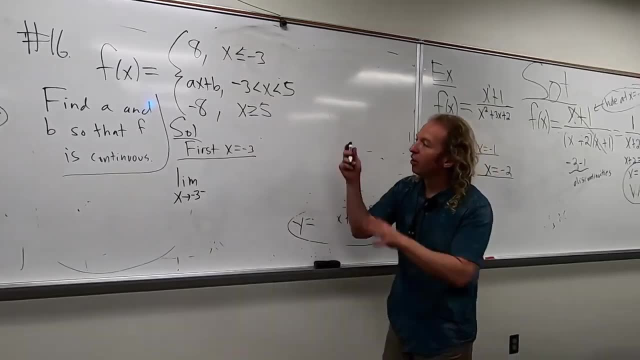 So take the limit from the left. So if you want to think of it in terms of steps, it's fine. Whenever you're doing these problems and you have less-thans and greater-thans, just do one at a time And then just take one-sided limits. 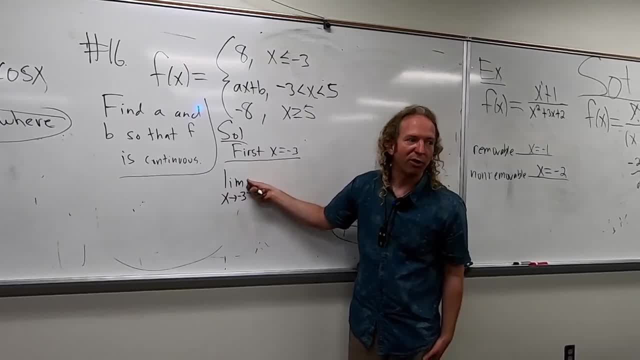 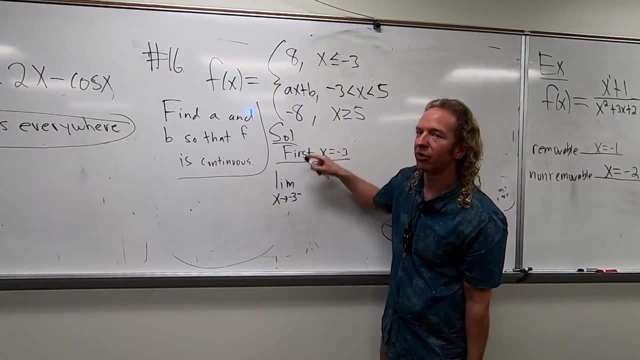 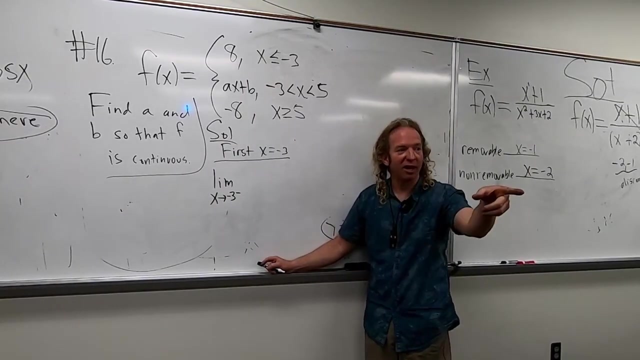 So the limit, So the limit from the left. So we have to figure out what goes here. So if we're approaching from the left, which piece do you think we use? Oh no, almost, Good try, 8. Yeah, why? 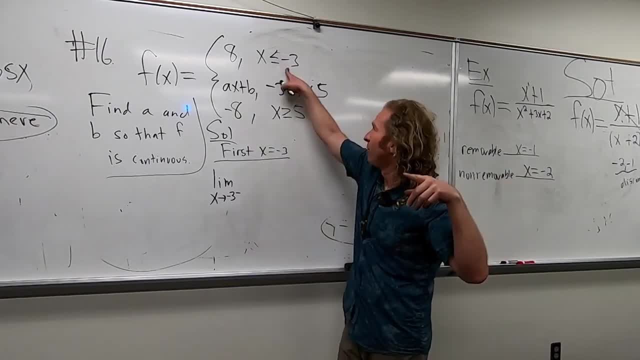 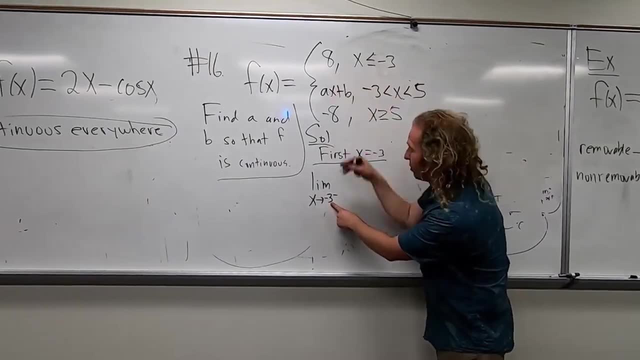 Why the top piece? Why, Very good. This tells us x is less than negative 3, right. So we're approaching from the left. So you want to use the top piece, So you put an 8 here. Everyone see that. 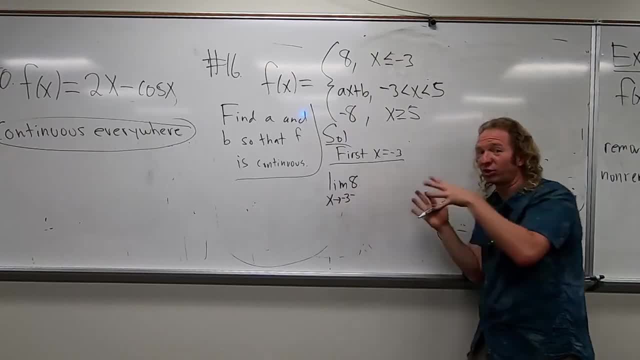 So because we're approaching from the left, we use the top piece, So you have to think It's a beautiful question. Again, this is considered hard. There's a bunch of easy homework, but we'll do that later. Good stuff. 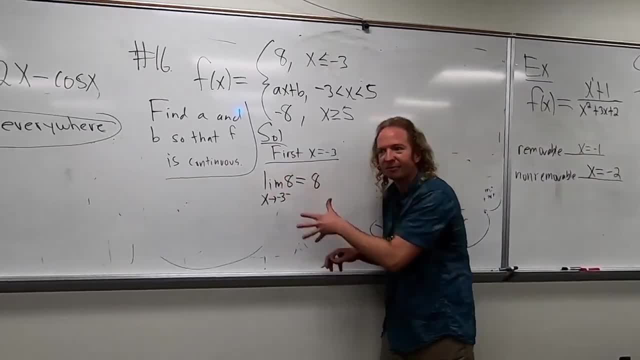 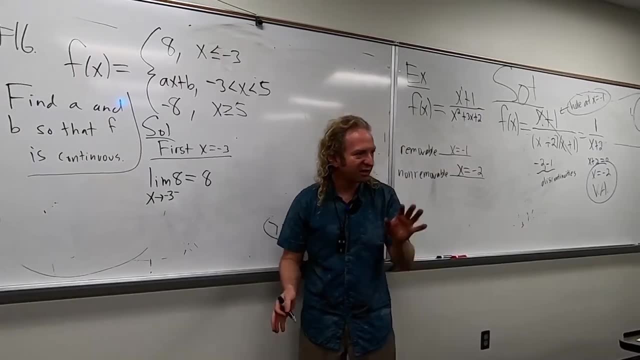 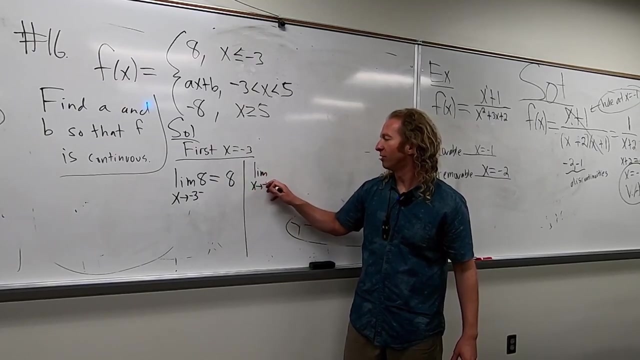 Easy limit, right, This is just 8.. So now you drop the limit. sign Good stuff. So now we have to do it again. Take the limit from the right. So I'm going to draw a little line here. So limit as x approaches negative 3.. 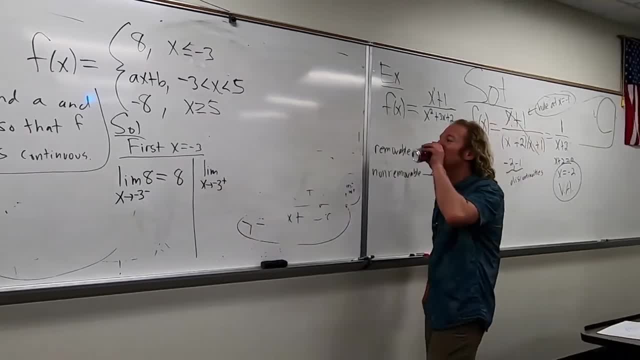 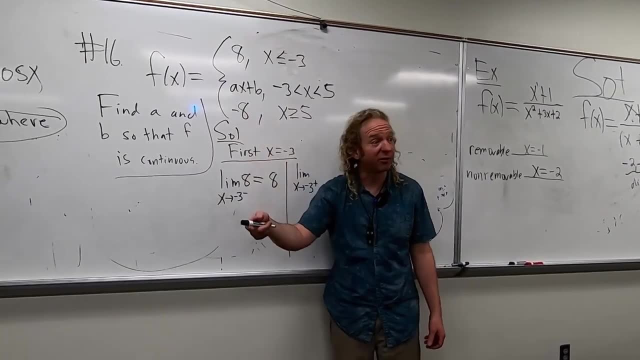 From the right. Which piece do you think we're going to use? First, second or third? Second, Very good. Some people might say, oh, but 5, that's bigger than negative 3.. You want to be really close to negative 3,, but bigger. 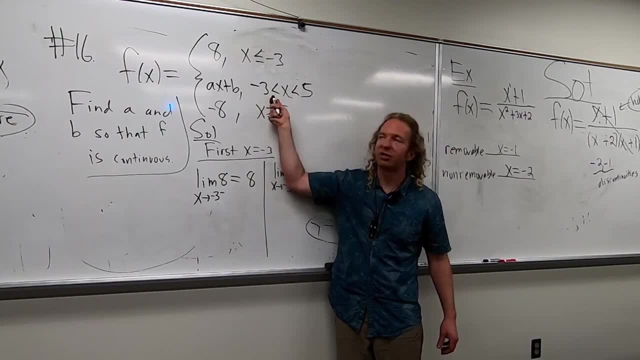 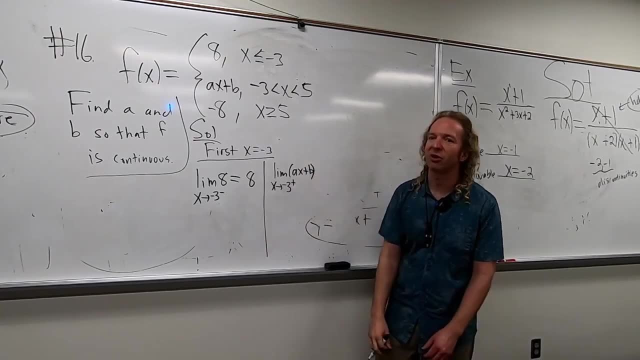 Read it backwards: x bigger than negative 3.. So the second piece. So here we're going to put ax plus b, Trying to go really slow because I know this is hard, It's pretty tough. So again, x is bigger than negative 3, right. 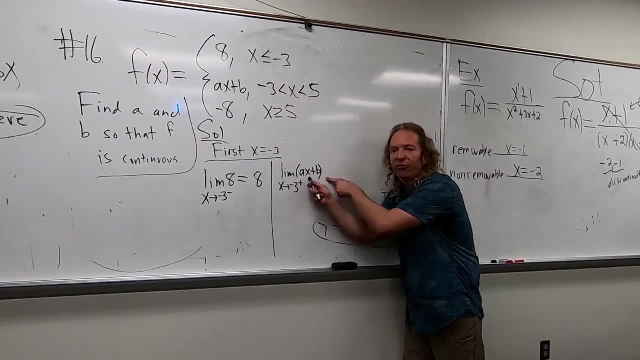 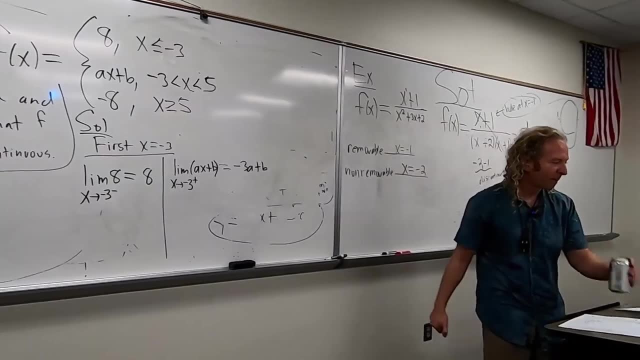 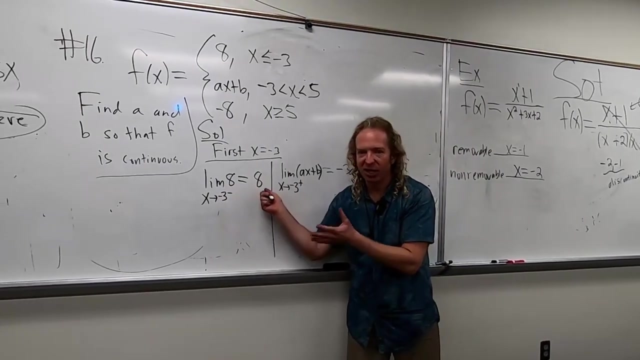 So we're coming from that. Okay, so now we can actually plug in the negative 3 for the x, So we get negative 3a plus b. Good stuff, All right. so the limit from the left is 8.. The limit from the right is this: 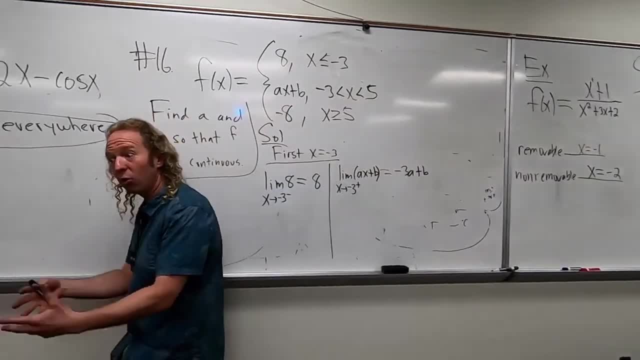 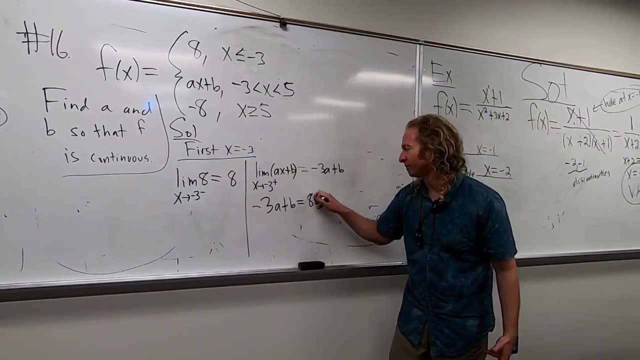 We want the limit to exist, So they must be. what Equal? Oh my God. Yes, yes, Yes, good. So you set them equal. Yes, very good. You set them equal to each other, right? Because you want the limit to exist. 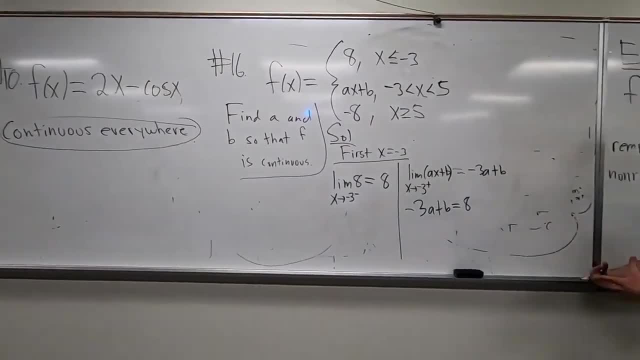 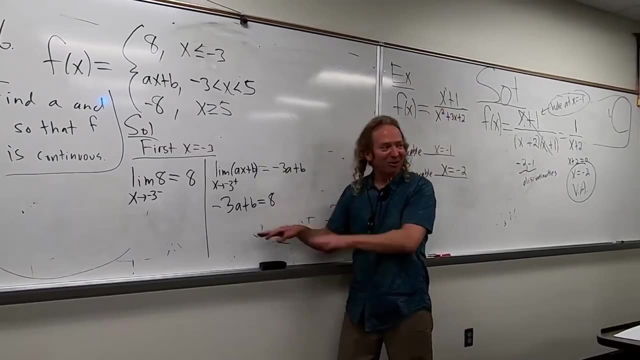 That's the idea, right? That's the concept. This is a really deep conceptual question, right? That's why it's considered difficult, right? I just got goosebumps. So that's the first piece. So now we're going to go to the second piece. 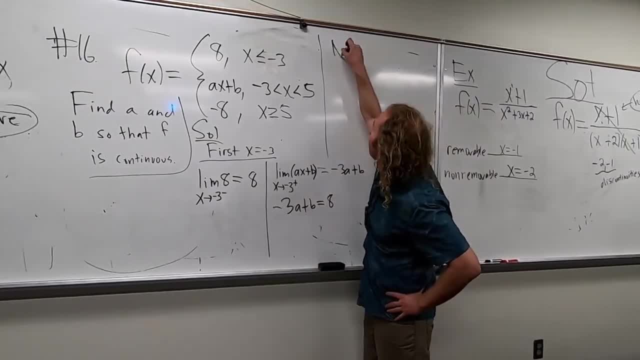 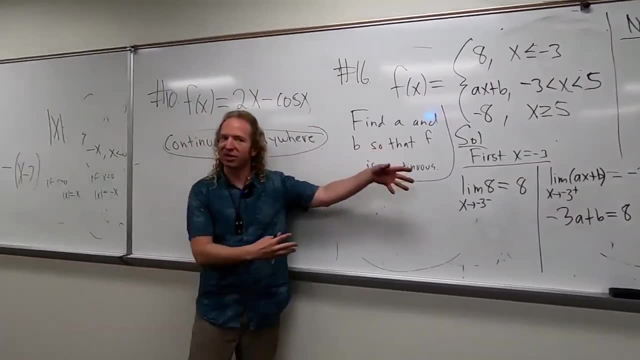 So now we have to do 5.. So now let's do 5.. So now 5.. Yeah, this is going to be Like if we had never done this in class and this was on a test. can you imagine? 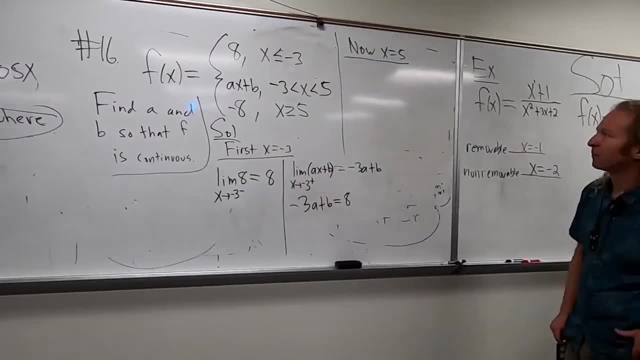 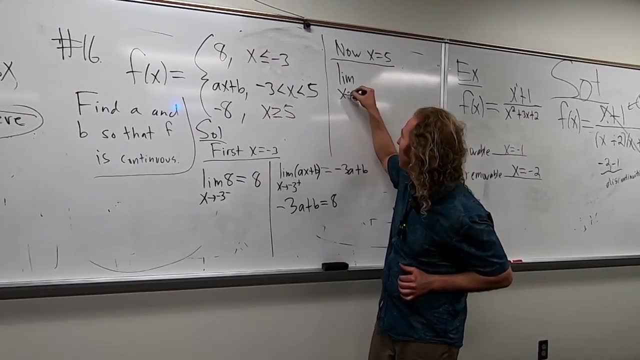 Like that'd be like really tough, Yeah, Okay, So let's take the limit from the left, Limit from the left as x approaches 5.. So which piece should we use when we're approaching 5 from the left? 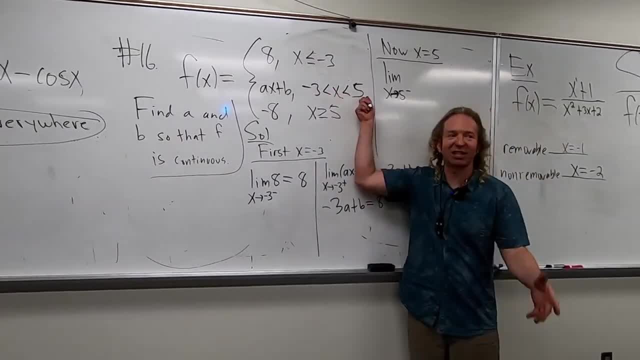 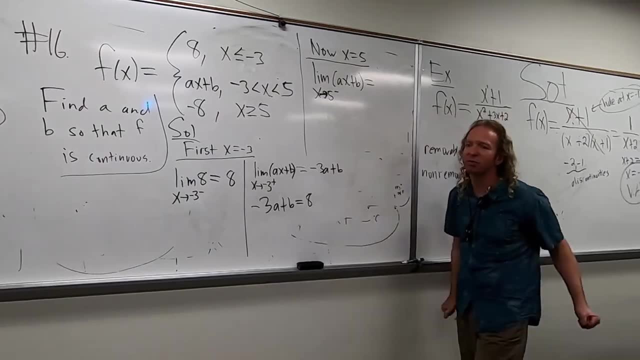 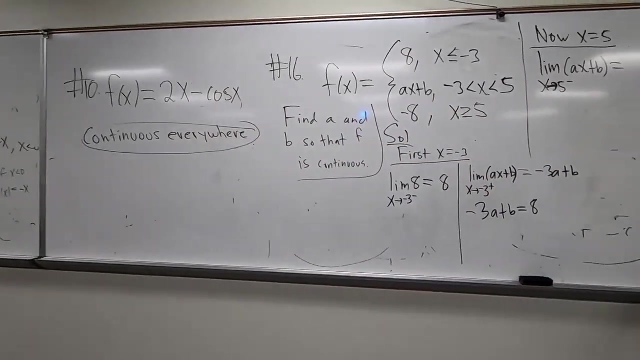 Third: Nope. Second Second: yeah, because x is less than 5.. Everyone see it Good, good, good. So ax plus b, Ax plus b, Ax plus b, Good stuff. And so now we replace the x with 5 and we drop the limit, sign right. 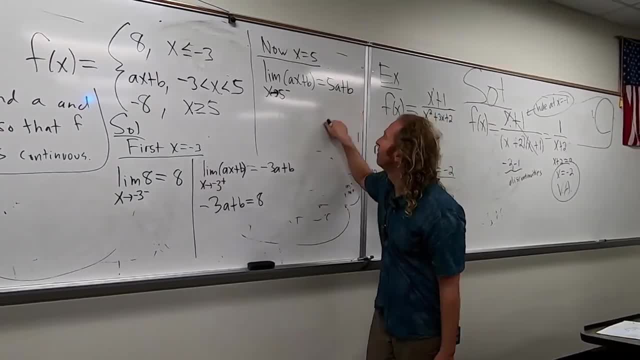 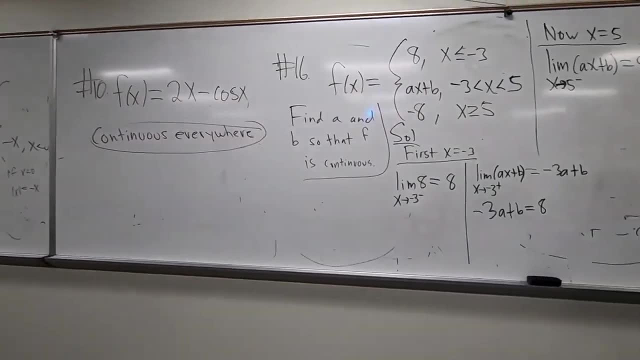 So it'll be 5a plus b, 5a plus b, 5a plus b. There's one on the worksheet like this: I think too. All right Now, we just got to do the limit from the right. 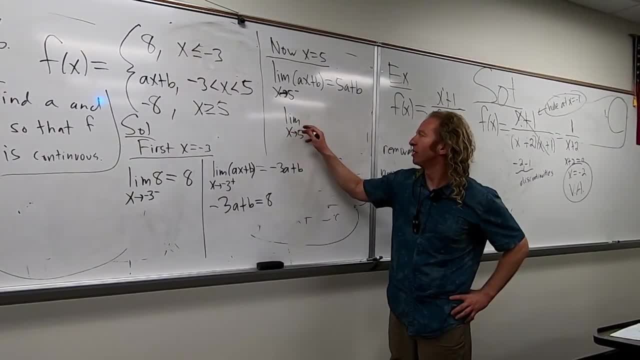 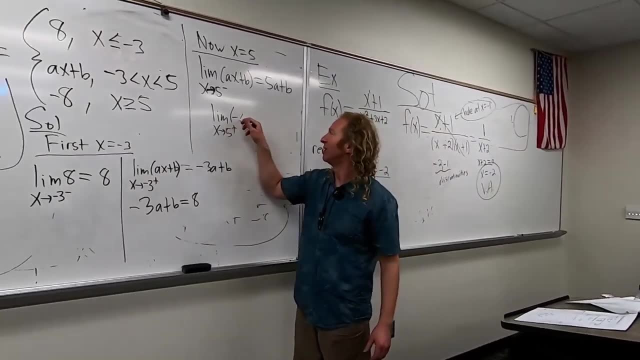 So limit as x approaches 5 from the right. What is it, Logan? Negative 8.. Yeah, negative 8.. Good, Negative 8.. So now you just plug it in and you just get negative 8.. Let's take a negative 8.. 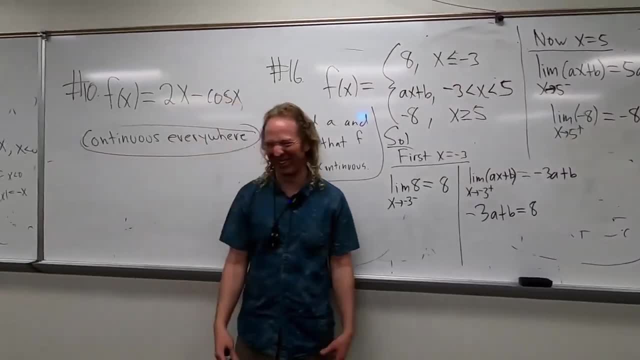 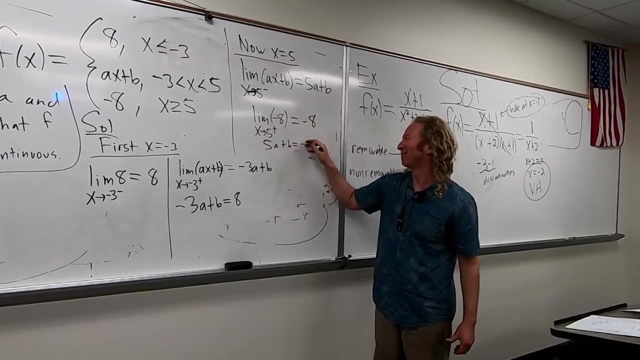 What do we do next with these? Set them equal. Set them equal. Oh, so good. I wish I could just give you a name, but I can't do that now. Like, oh, eat the nose, Like that's it, you know, but no, can't, can't. 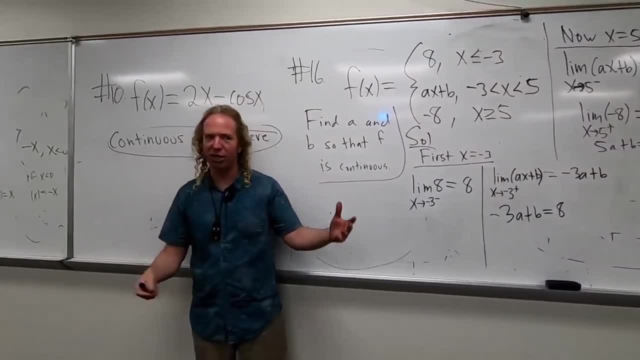 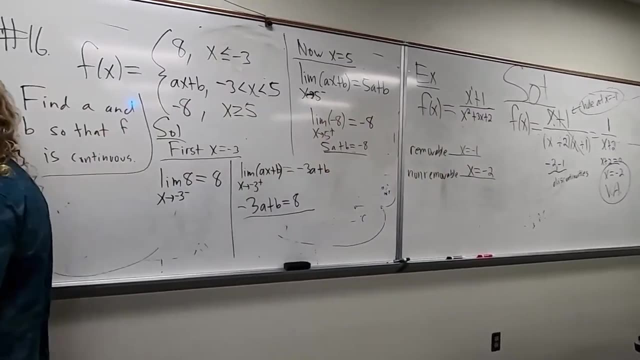 Yeah, I wish it was that way. Like there was no test, Like you would, just you got it in class. so, like you know, Okay Someday. So we have two equations. We have to find A and B, so I guess we can solve them right. 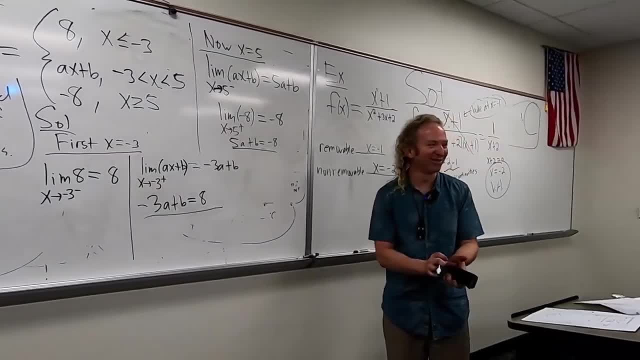 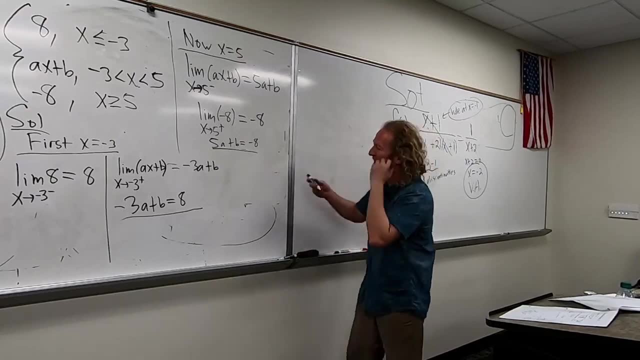 Let's use Kramer's rule. No, I'm kidding, I'm kidding. No, Do you remember Kramer's rule? Let's just solve it like a normal way, Like how humans put it in a matrix. No, it's, I'm just going to write them above each other. 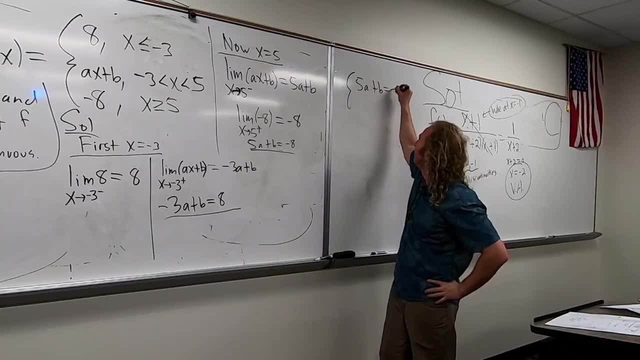 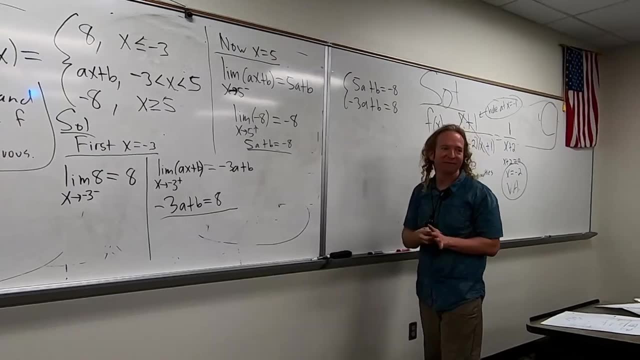 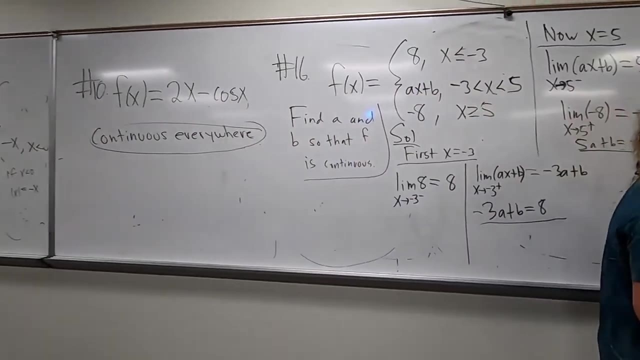 So if 5A plus B equals negative 8, negative 3A plus B equals 8, equals 8, we have to solve the system of equations. We could use substitution. I guess It might be easier to just maybe multiply 1 by negative 1.. 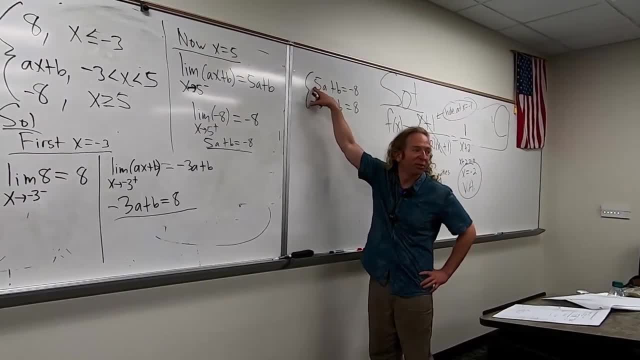 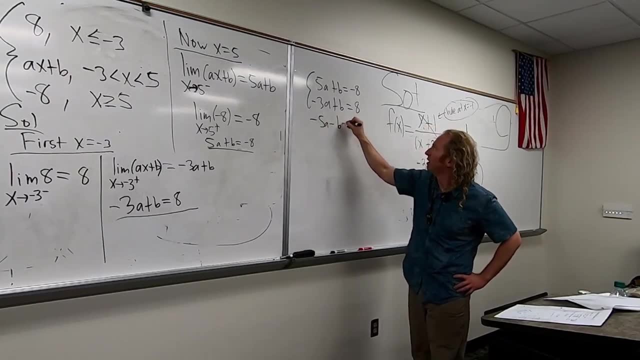 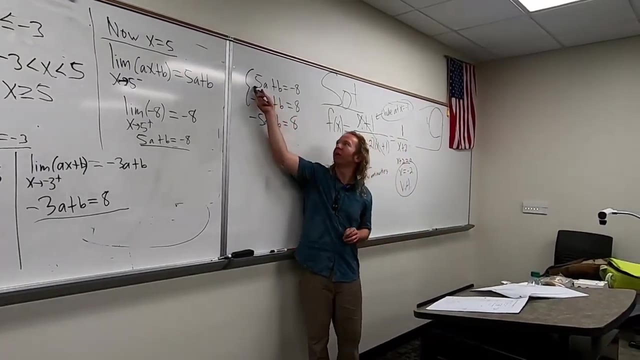 I'm going to multiply the first one by negative 1.. So, multiplying the first one by negative 1, we'll get negative 5A minus B equals 8.. Did I do that right, 8.. Yeah, multiplying the first one by negative 1, negative 5A, negative B, positive 8, positive 8.. 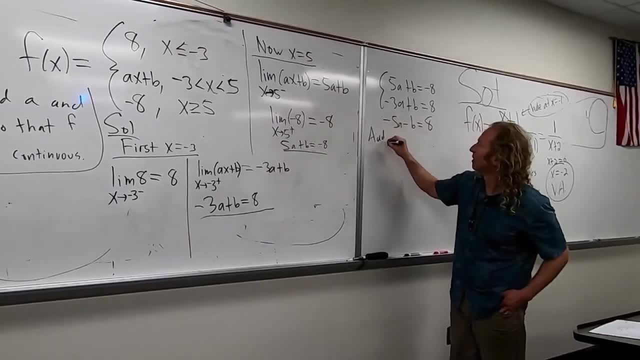 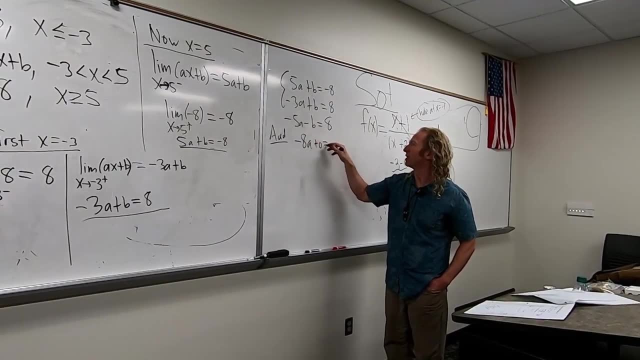 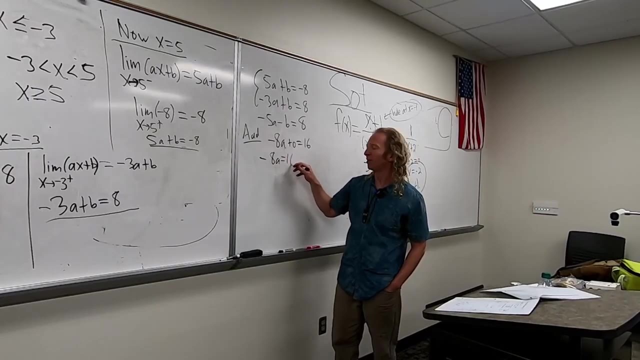 And then we can just add them. right, We can add now, So we get negative 8A. Adding the B's, we get 0 equals 16.. Oh, this feels really good, because now we get a really pretty answer, right. 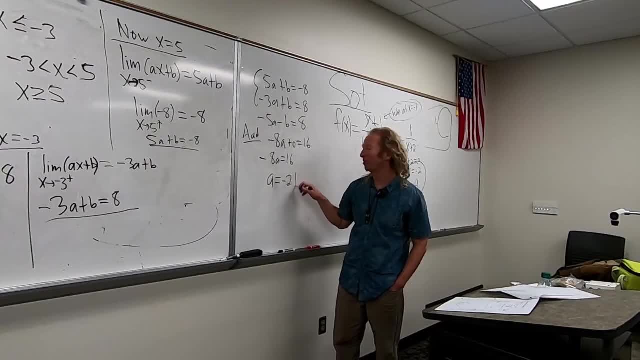 We get A equals negative 2.. Yeah, really nice, right. It makes you feel like you're doing it right, Like, ah, you get negative 2 on a test. You're like, yeah, You know you got it right.